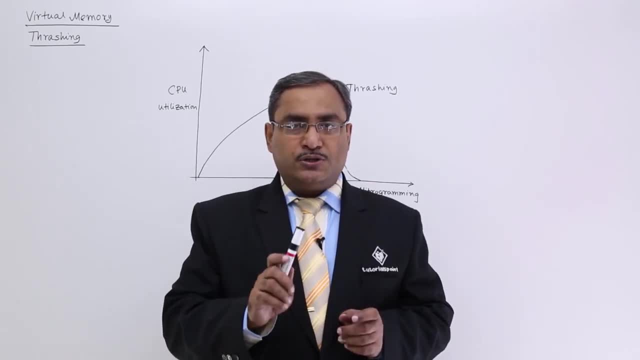 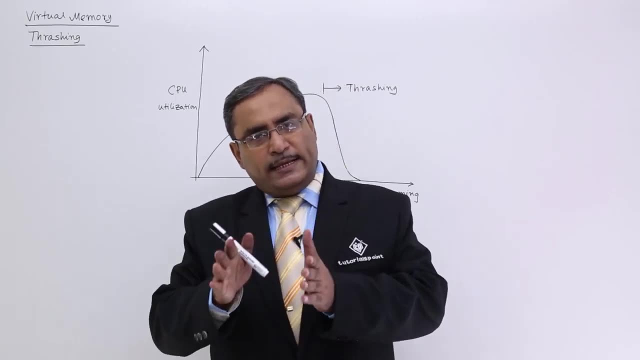 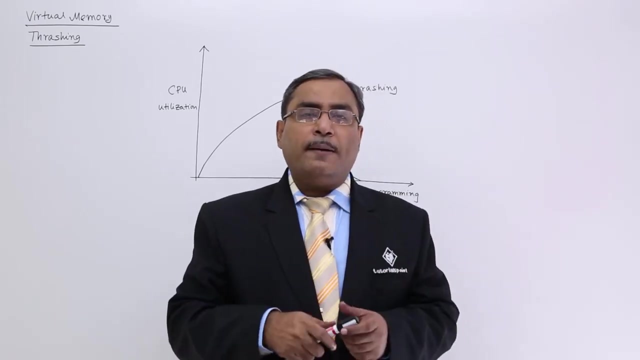 in my previous example I had 5 frames. So if I increase the degree of multi-programming, that program will be allocated to 4 frames. If we increase the degree of multi-programming more than that, then it might be getting allocated for 2 frames. Then what will happen? All the 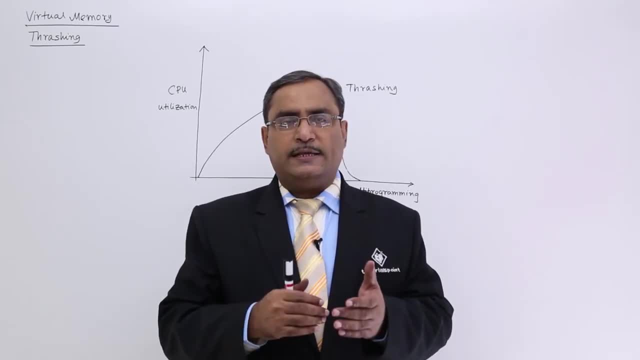 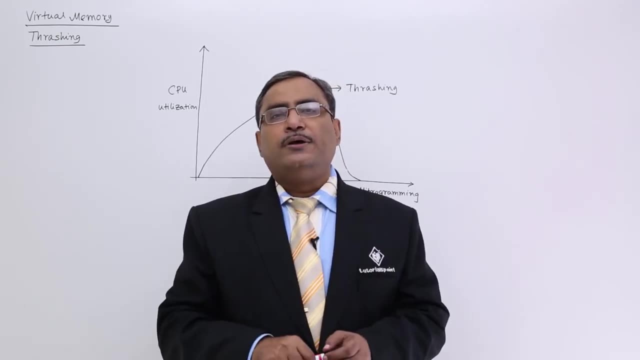 programs. during execution, they will face a page fault. The page fault occurrence probability will be drastically high. So what will happen? The system will be busy, not for execution of the program, but for paging. This situation is known as thrashing. Now why should I increase the degree of multi-programming? Because if I increase the degree of multi-programming, then in that case multiple programs will be existing inside the computers memory. so the probability of finding a particular program requiring cpu will be enhanced. and if always cpu can keep itself busy finding a program from the memory which is requiring its interaction, then the cpu utilization will be high. so obviously, 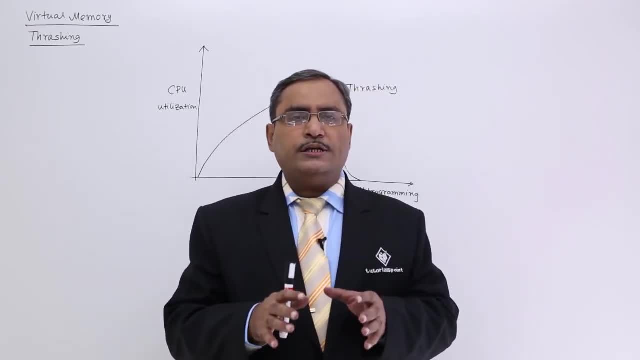 we should have an have an aim to make the cpu utilization maximum. but in this process, if i go on decreasing the number of frames allocated to each and every process and and if the processes are not getting minimum or optimum number of frames for their execution, then during that execution they will cause page fault as a result of that. the system. 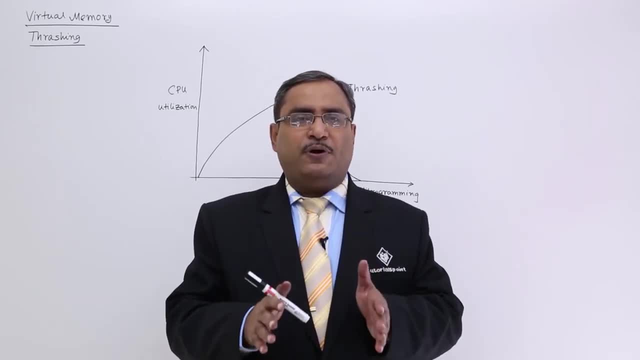 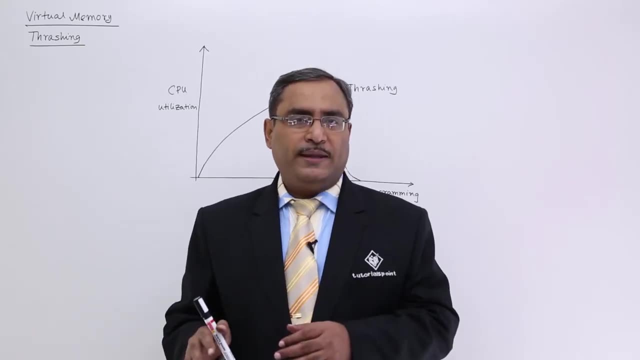 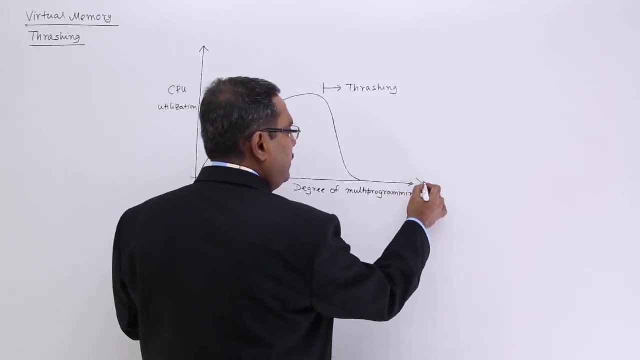 will be busy for paging, for paging Page faulty Page faulty page fault handling, not for execution- then again the CPU utilization will be drastically drop down. and that has been depicted in this particular graph. Along the x-axis we have plotted degree of multi-programming. Along the y-axis we have plotted CPU utilization. So if we go on increasing, 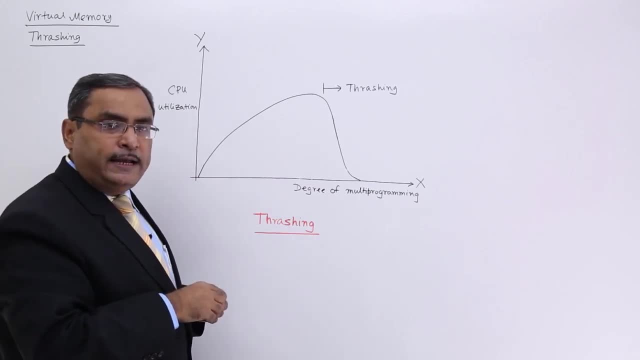 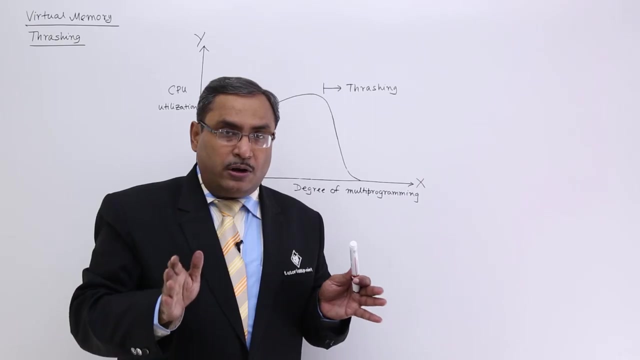 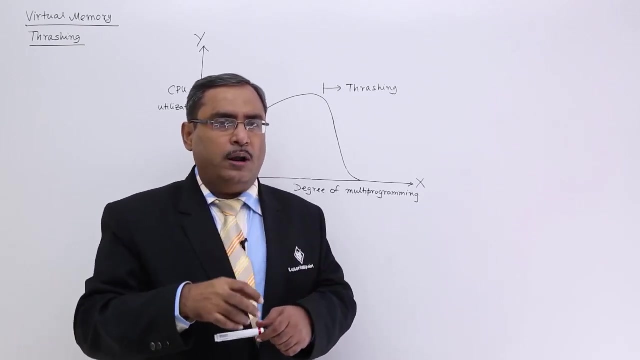 the degree of multi-programming, the probability of finding a process existing in the memory requiring CPU execution. CPU processing will be high, So the CPU utilization will be enhanced. but if you are not processing memory, you are not installing new memory within the same amount of physical memory. you are going to increase the degree of multi-programming. Then what will happen? 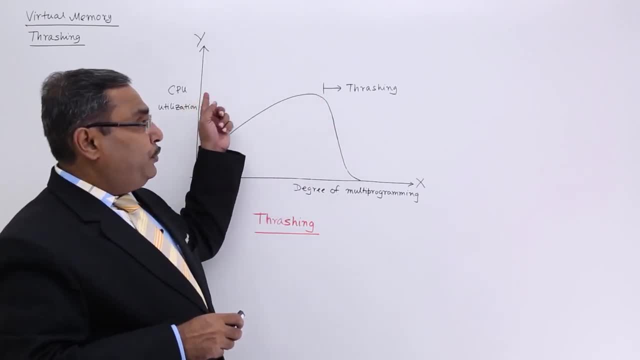 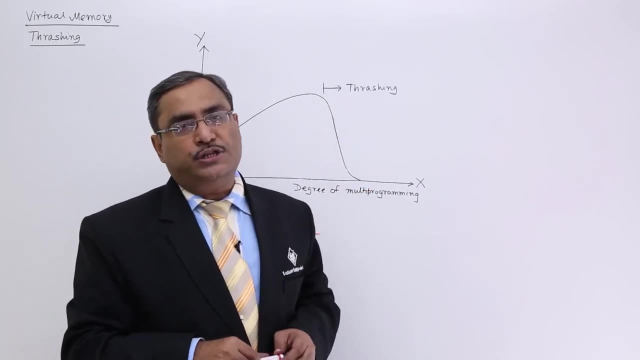 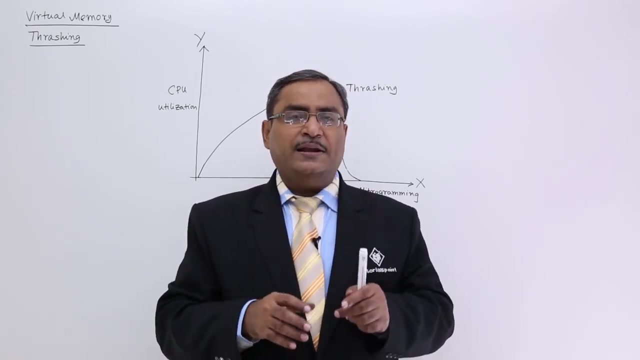 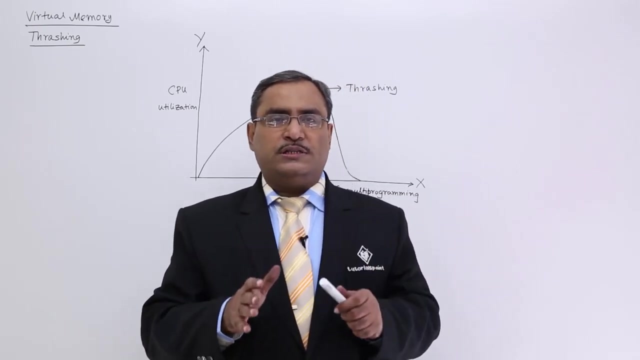 after some time, this particular CPU utilization will be drop down in a very sharp way and this phenomenon is known as thrashing. So what is thrashing means? thrashing means high page fault rate and drastically reduction of the CPU utilization. So obviously a process requires optimum.